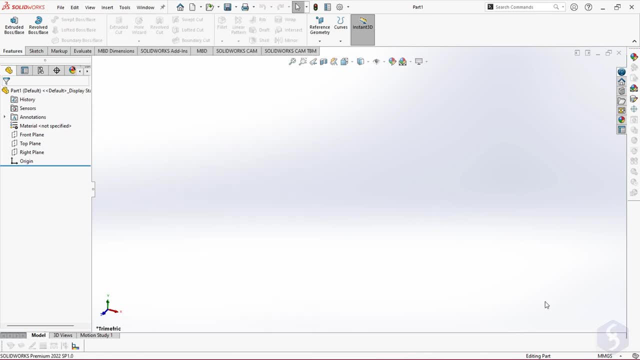 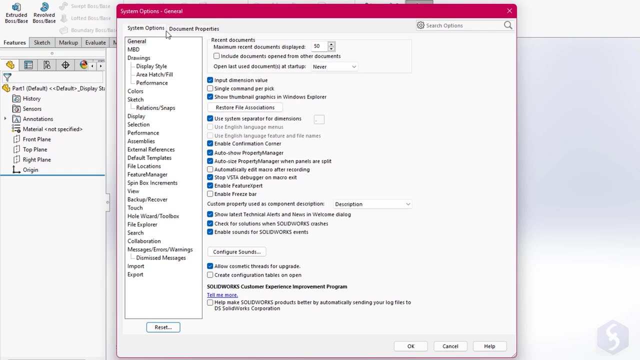 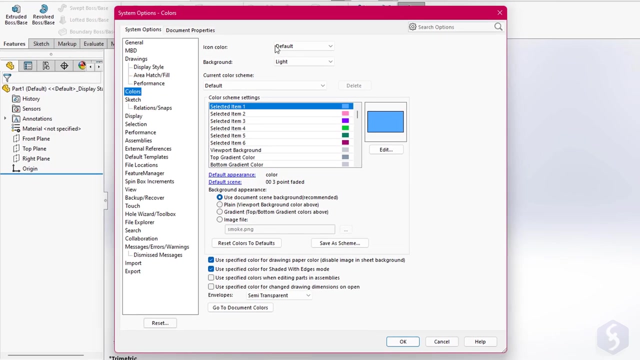 At first you may need to set the main project properties, such as the units to use. Click on Options on top to adjust either the basic system or the document properties specific to your current project. For example, on System Colors, you can choose a dark theme for the general interface. 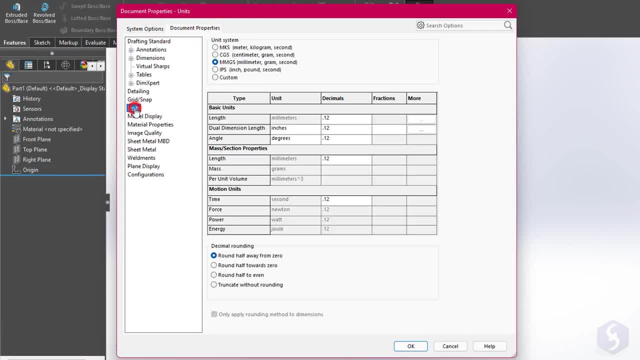 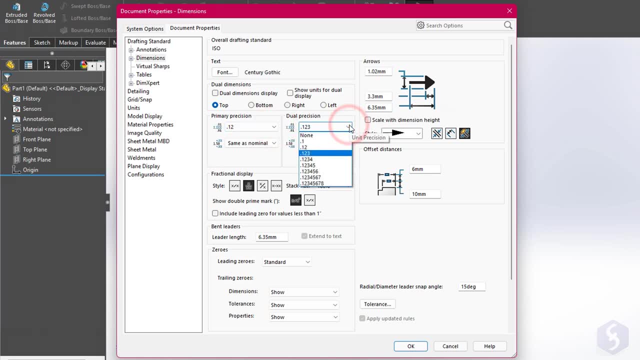 On Document Units, you can adjust the units to use And on Dimensions, you can set how to show measurements and detail. At this point you're ready to start drawing. In a Part project. you can drop 3D objects called Features. 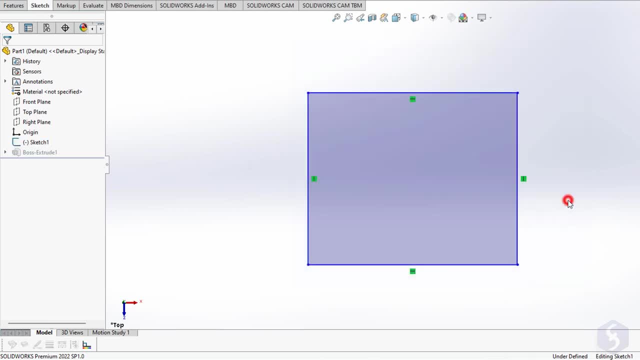 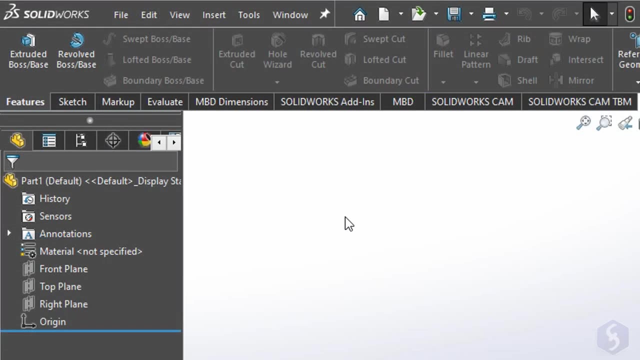 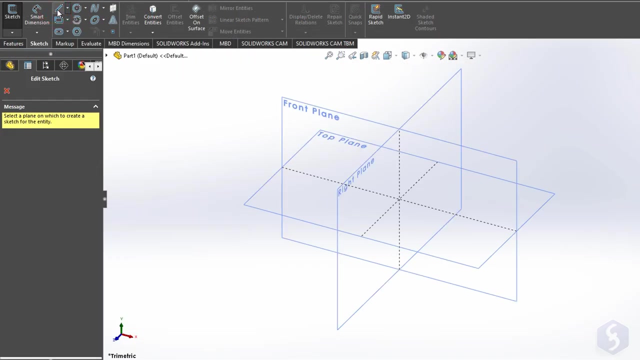 and 2D drawings, called Sketches, Starting from elements like lines and curves called Entities. Let's start making 2D drawings. From the Sketch section on top you find all the tools to 2D draw. The first time you enable any tool. you have to choose the plane to draw on. 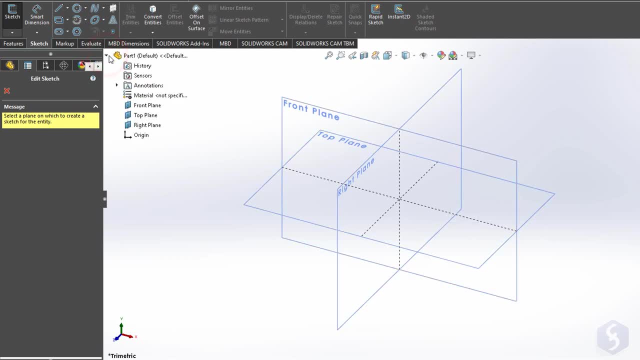 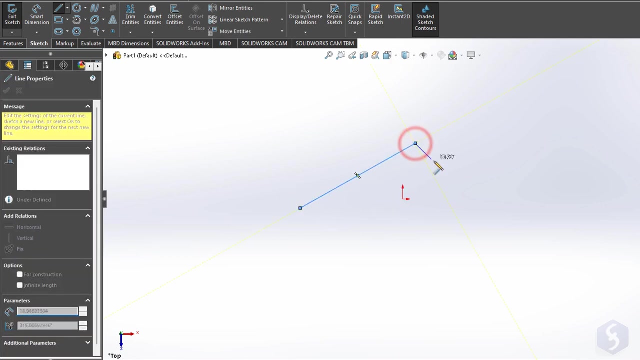 From either the Preview or the Quick Selection list on the left. we suggest to always draw 2D objects on the top plane, which represents the ground plane. At this point you can start drawing With the Line tool. you can drop consecutive straight segments by clicking multiple times. 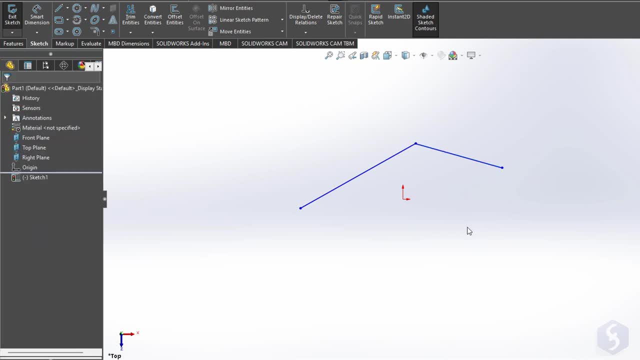 using the Escape key to stop drawing, Use the Enter key to always recall the latest tool and draw again. With the Spline tool, you can draw a spline curve by fixing several nodes, double-clicking on the last one to apply, Whereas use the Arc tool to drop an arc with two points for the radius. 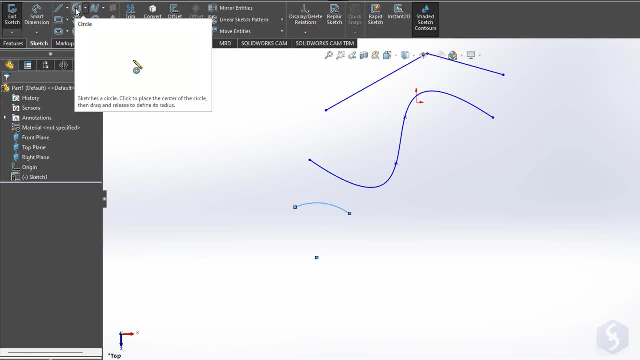 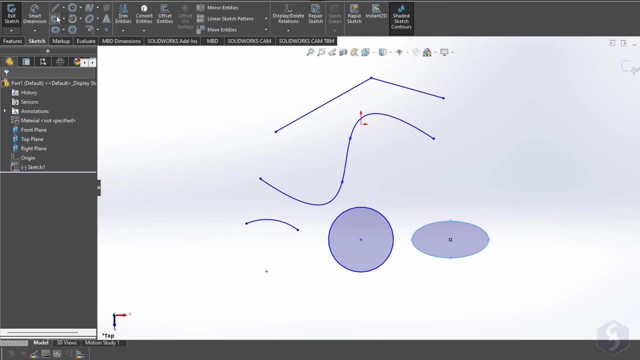 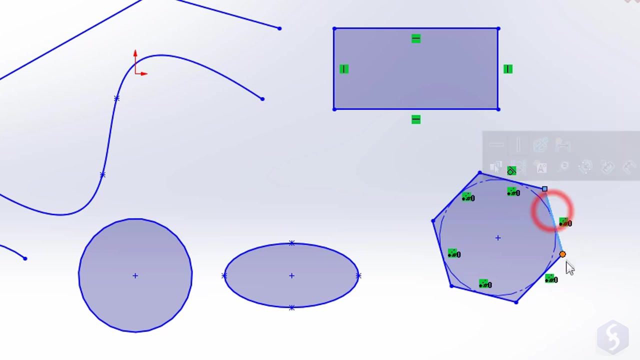 and another for the arc length. Enable the Circle and the Ellipse tool to drop circles and ellipses with two or three points, Whereas use the Rectangle and the Polygon tools to drop regular shapes by clicking twice. Consider that all rectangles and polygons are simply groups of straight segments combined together. 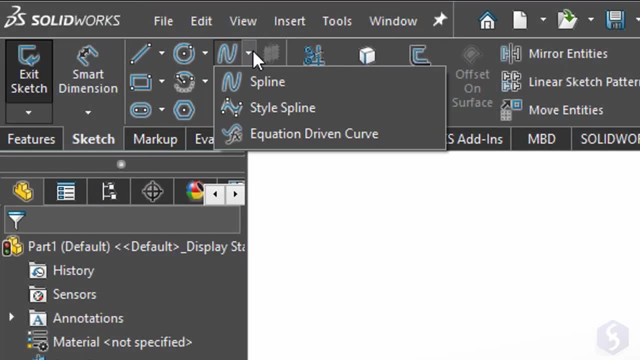 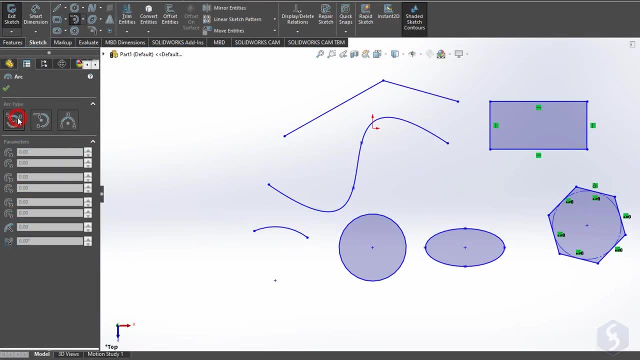 Each 2D tool includes other drawing modes. under the down arrow, You can hover over the main button to get useful tips. Furthermore, the Property Manager on the left allows to change the drawing mode as well as the drawing properties, such as the sides of a polygon. 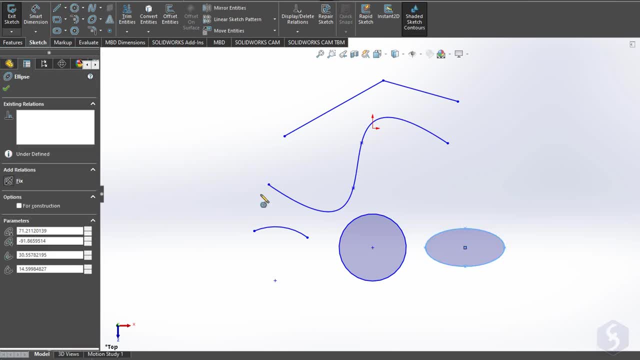 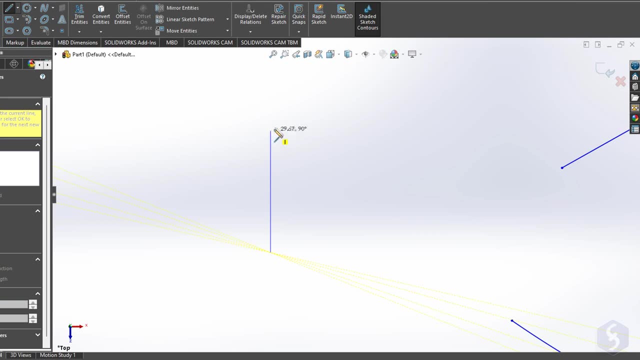 Remember to use Control and Z to undo your latest actions. Solidworks has several drawing aids. While drawing, it shows live measurements on length and radius, as well as dashed guidelines to follow perpendicular or tangent directions. You also get snappings to object key points, like endpoints. 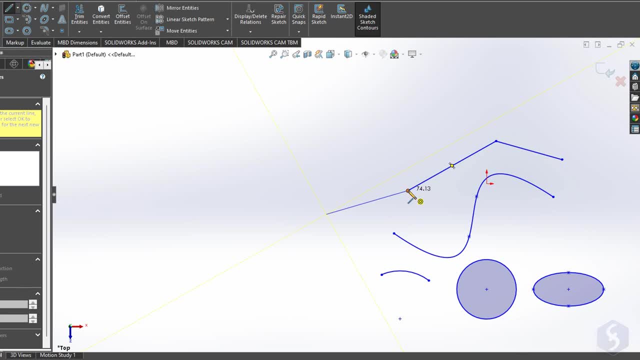 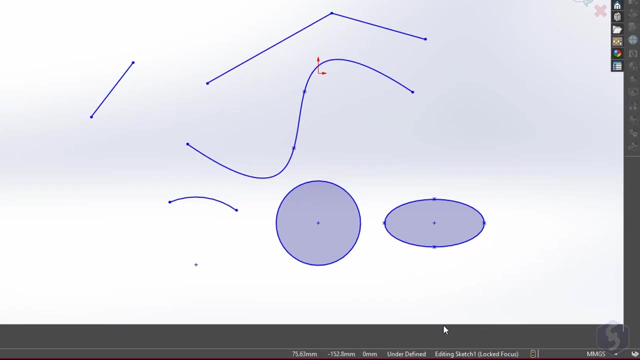 midpoints and centers that you can disable by holding down the Control key. Special symbols on your cursor or on sides show the kind of relations applied on such entities. All drawings made are part of a single 2D sketch called Sketch 1,. 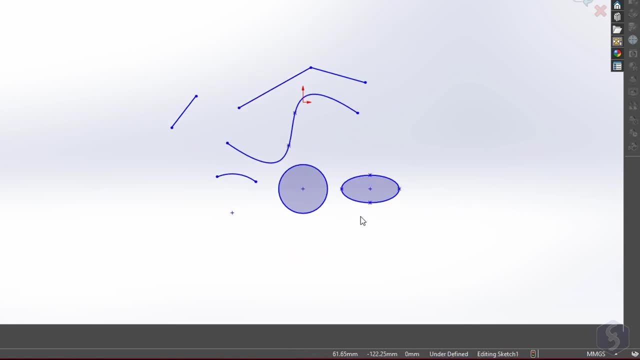 as you can see at the bottom, You can check these by zooming in and out with your mouse wheel and moving around with the arrow keys while holding down the Control key. To apply this sketch and exit from it, use Control and Q. 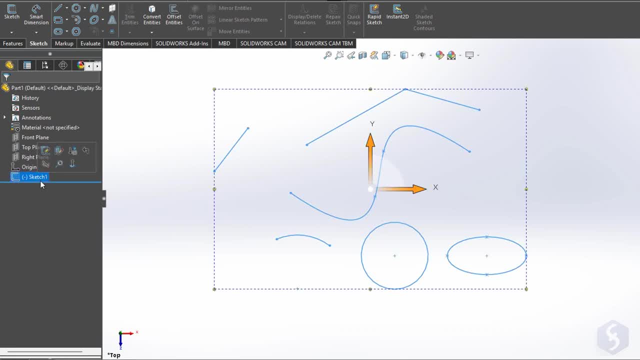 At this point you can select any sketch from the Feature Manager to move it with the arrows or scale it with its nodes. You can also right-click on it to go to Delete, to remove it or as to go on with a new 2D sketch. 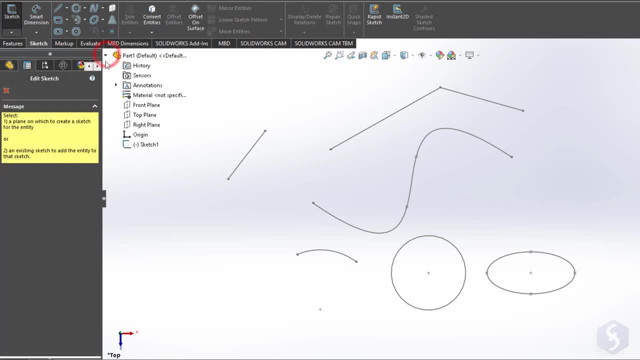 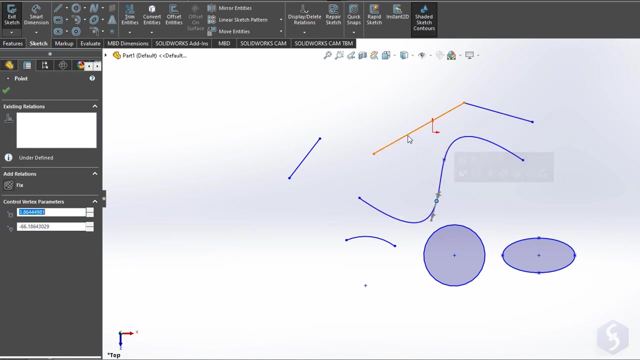 exit from any and draw with any tool, selecting the right plane again To edit existing drawings. double-click on any sketch to enter it first. With no tools enabled, you can use your cursor to select points, lines and curves setting their options from the Property Manager on the left. 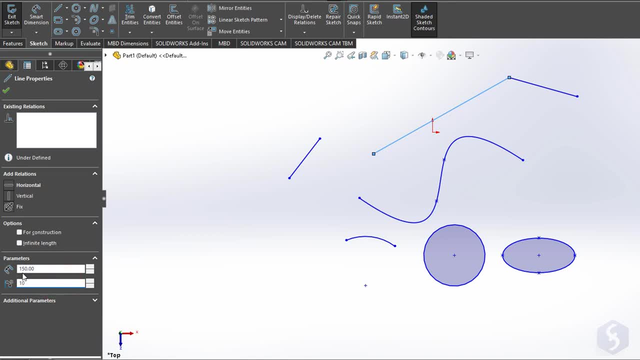 These include relations, length, inclination and center positions according to the entity's settings. You can cut, copy and paste a selected entity with Control and X, C and V Cut any entity to remove it in no time. You can drag any node to move it. 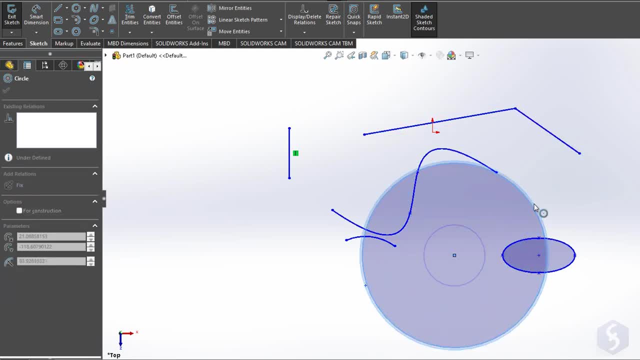 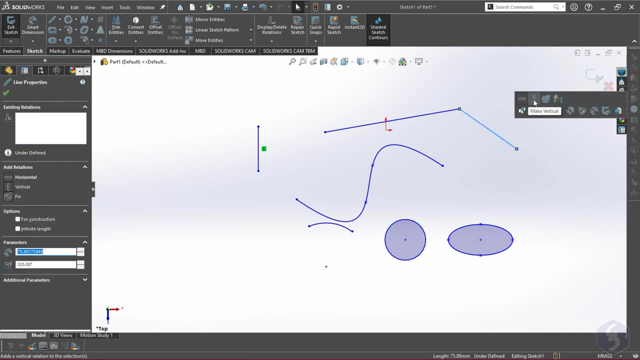 or any side or circle to adjust length and radius. From the dialog box you also get additional options such as horizontal or vertical, to make any side parallel to main directions with a proper relation, or construction geometry to turn the entity into a guideline for your next drawings. 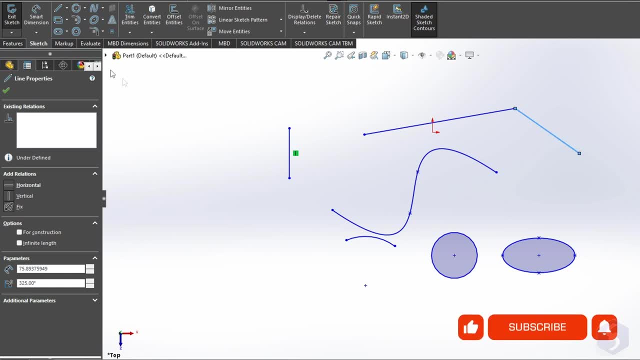 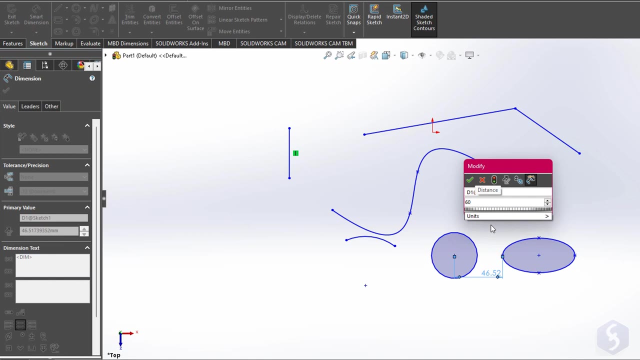 With SolidWorks, you can also make precise drawings while using your keyboard. If you enable Smart Dimension on top, you can select points, sides and curves to drop useful annotations on any distance, length or radius, but also correct them on the go by typing in. 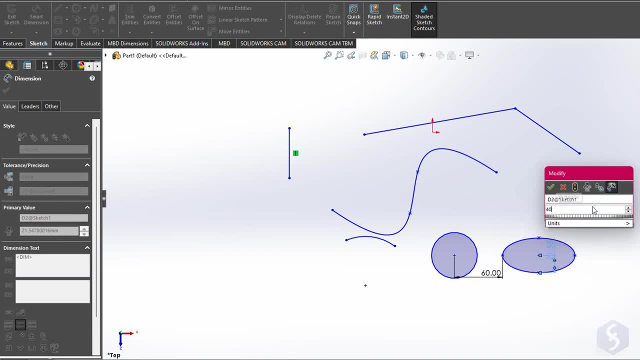 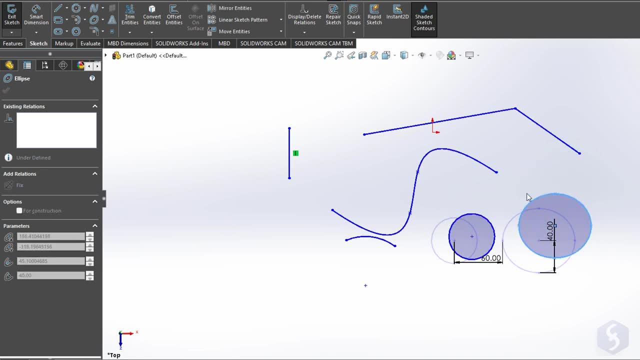 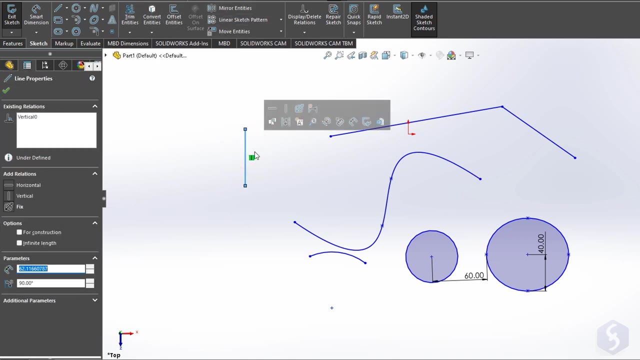 and applying with the Enter key. These annotations also move and edit entities in order to respect their relation. From the Sketch section you also have advanced 2D tools. Select any entity and enable Move Entities to move it without changing its properties. 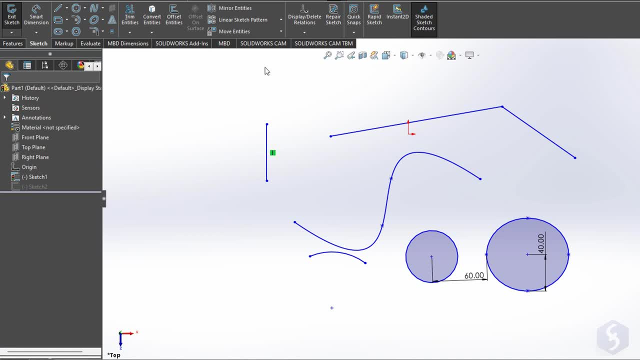 right-clicking to apply. These tools can also be applied to groups of entities. Click and drag on it to select all of its sides or select each one while holding down the Control key. At this point, you can enable Rotate Entities, Define the center of rotation and then rotate the group. 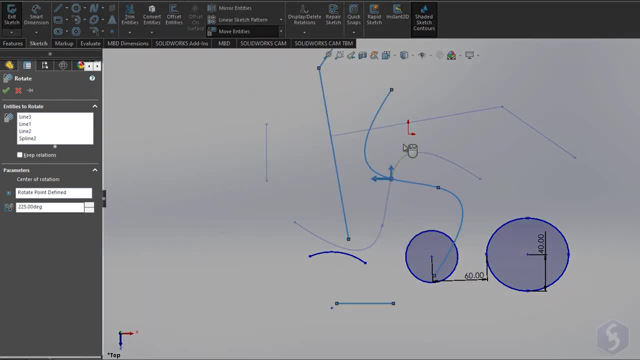 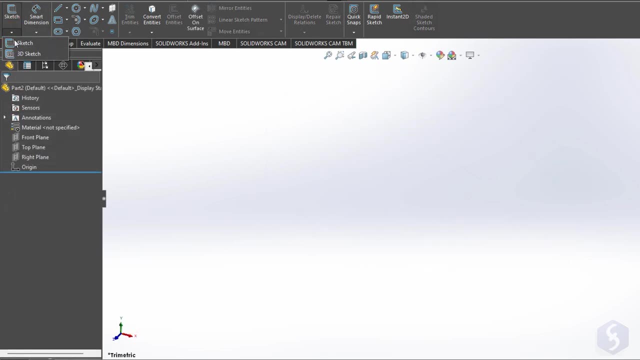 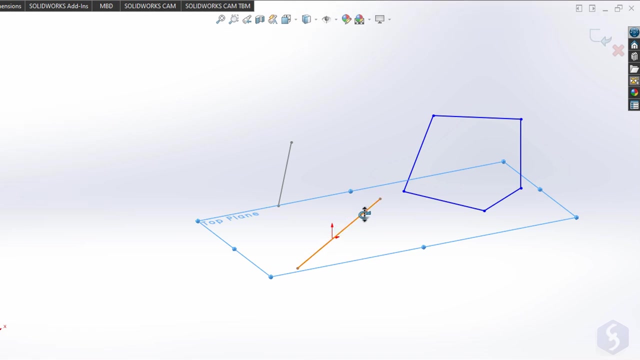 Always check the entity selected on the left and all relations applied to them in case the tool does not work as expected. Besides 2D sketches, you can drop 3D sketches to draw 2D entities in a 3D environment. These differ since 2D sketches physically lay on a single plane. 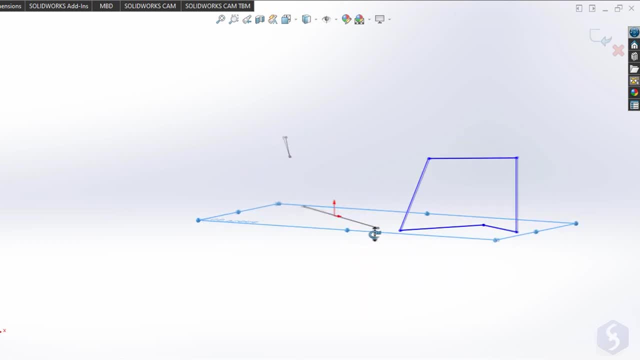 whereas 3D sketches can be drawn on a single plane, They can be parallel to any plane or even spread towards multiple planes. The way to draw 3D sketches is identical to 2D ones, enabling any drawing tool and selecting the right plane. 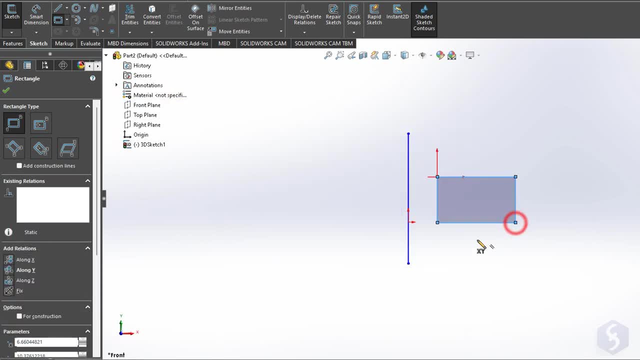 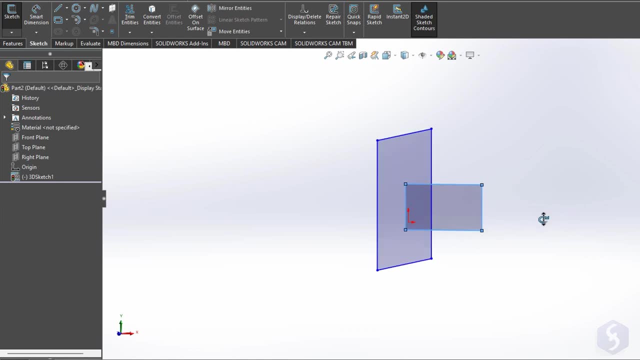 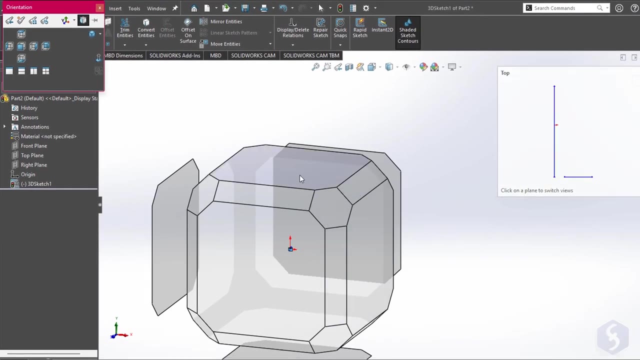 You can always change the plane to use by selecting it and going to Normal to. To get a complete 3D preview, right-click, go to Rotate View and click and drag around using the Escape key to exit. You can also use the Spacebar key to select specific views. 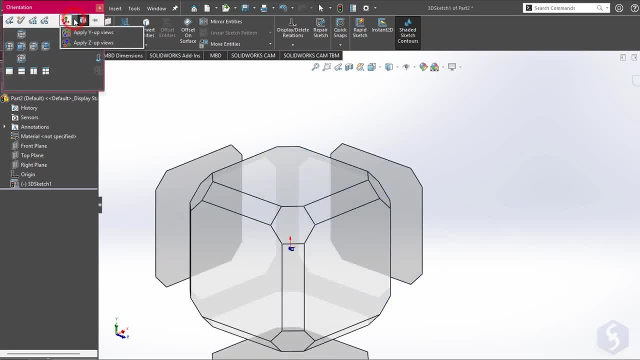 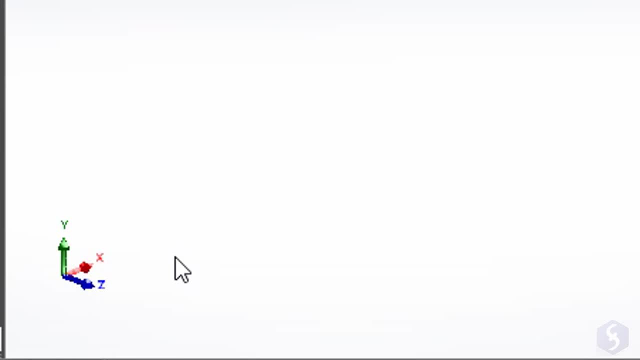 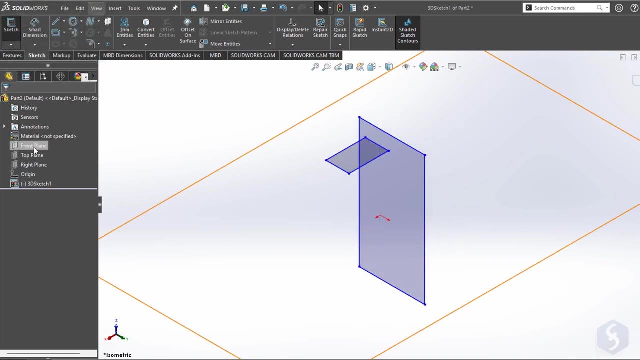 From the Orientation dialog. you can also change the coordinate system. By default, SolidWorks uses XZ as ground plane and Y for depth, but you can switch to XY and Z for depth. Pay attention that this won't change the existing planes you have. 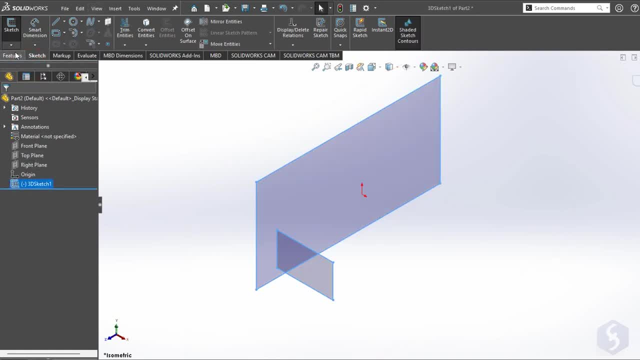 If you are in 3D view, you can only draw 3D sketches. In this case, the cursor shows the reference plane that can be changed with the Tab key. Always use CTRL and Q to exit the sketch and enable another tool to make a new, independent 3D sketch. 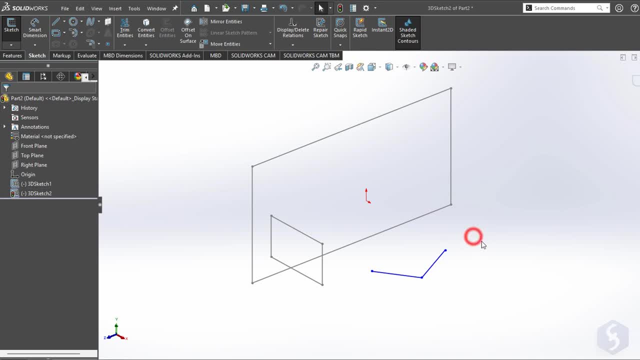 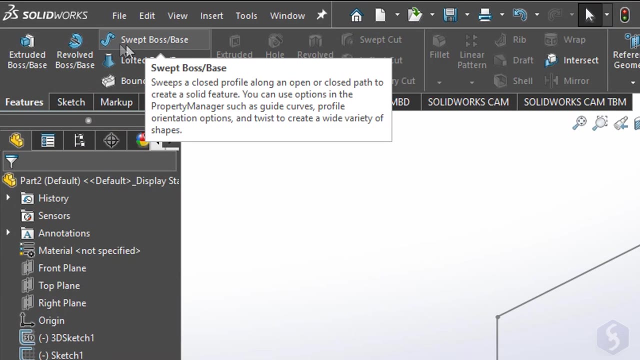 You can edit the entities of 3D sketches in the same way, with some additional options to make relations and additional axes when you move or rotate these. Now let's build 3D objects. On the Features tab you will find several tools to build 3D objects from 2D entities. 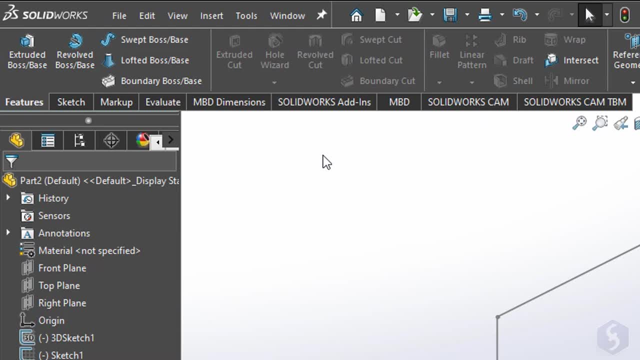 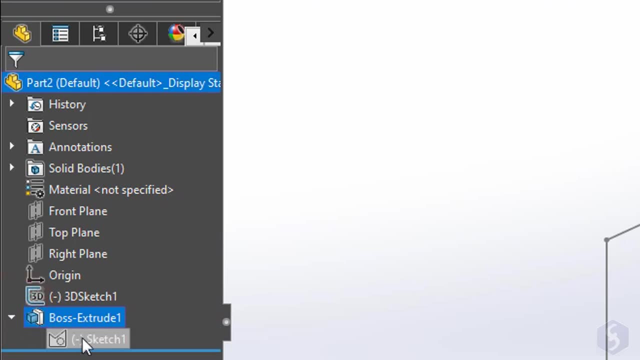 That can be either 2D or 3D sketches, depending on the tool. Pay attention that these sketches become part of the new 3D feature object, so make sure to dedicate an independent sketch per each new feature you are going to make. 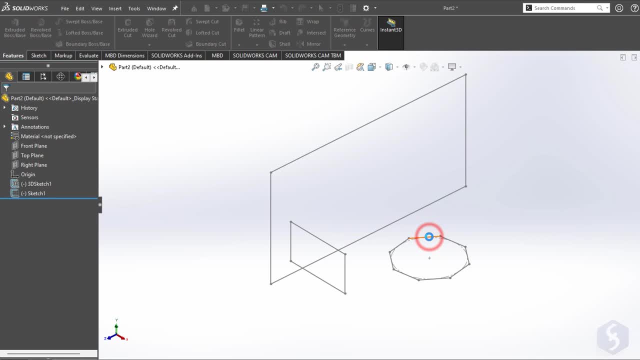 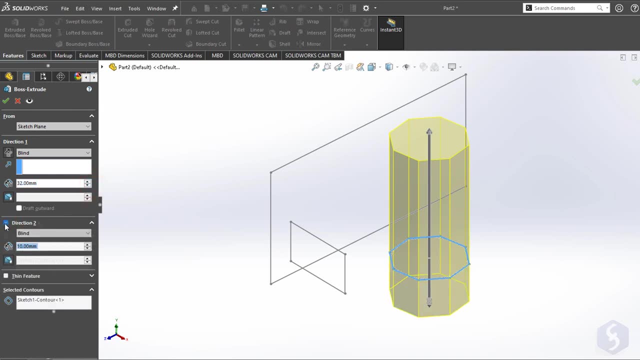 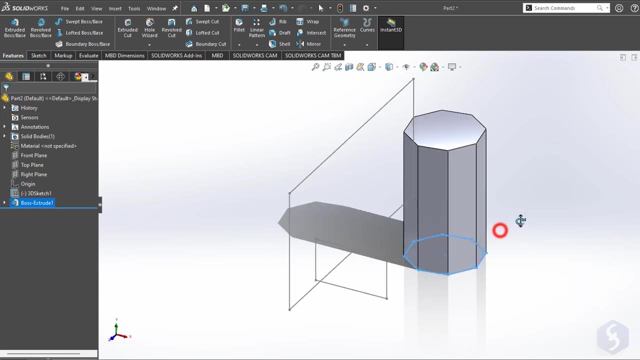 Enable Extruded and select a 2D sketch entity to add extrusion to it, adjusting proper options on the left. Then right-click or use the green checkmark button to apply. The 3D feature built shows some effects, such as shadow and reflections. 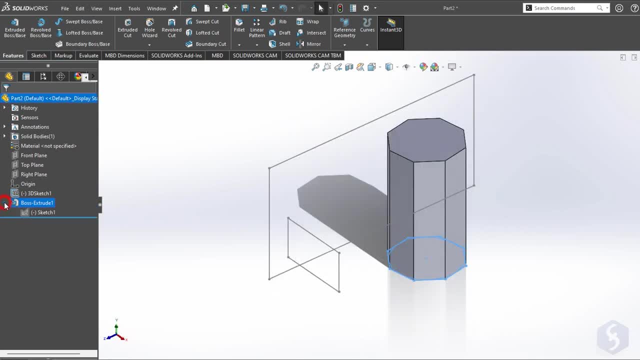 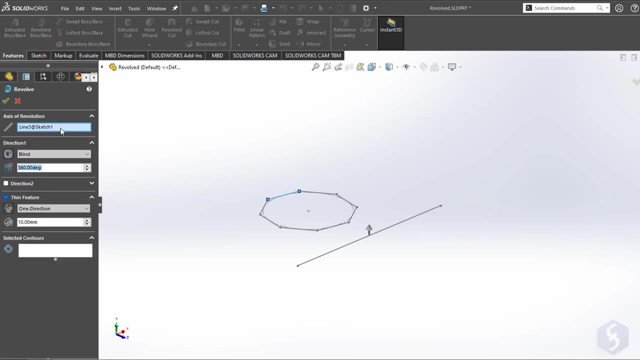 The 2D sketch used becomes a sub-component inside the 3D feature, but you can always edit it as seen. The 3D feature simply gets updated according to your modifications. Enable Revolve: to build a 3D object by revolving a 2D section around an axis. 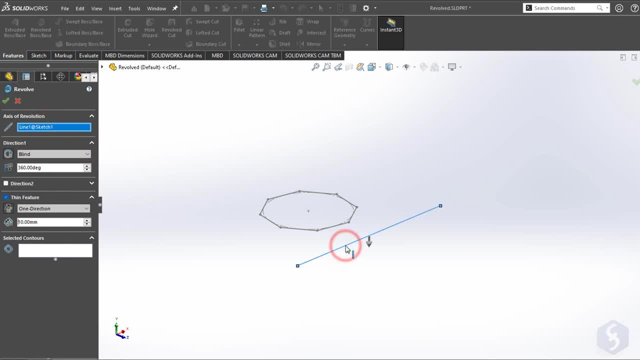 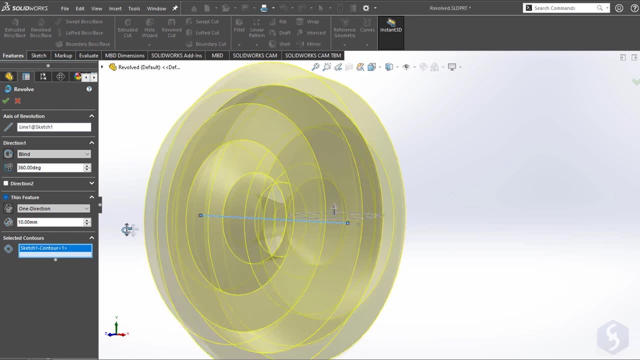 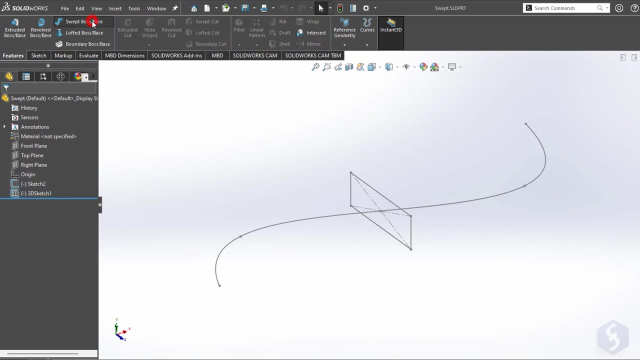 Click on Axis to select any line to use as axis. Then click on Selected contours to select the 2D entity to revolve. Make sure to adjust properties and degrees. from the left. With Swept you can build tubes and conductors. Click on the blue slot to select the entity to take as section. 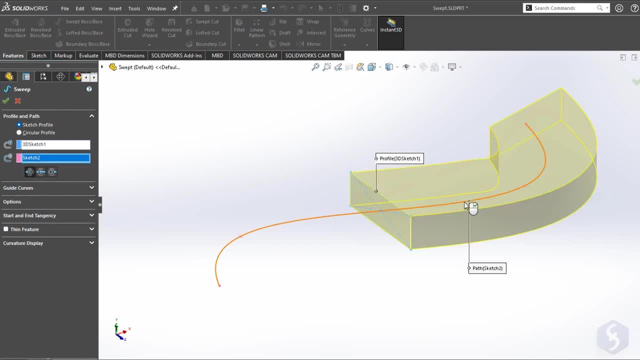 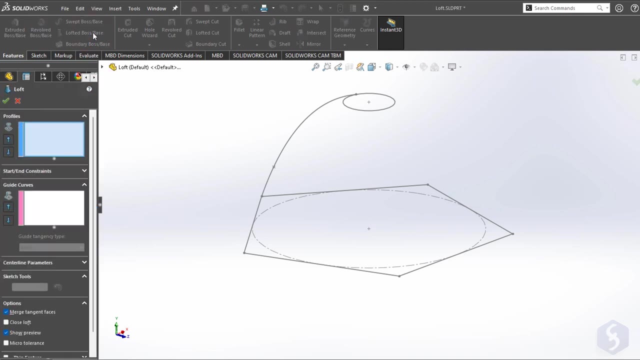 and on the pink one to specify the conductor path. Make sure that the original section is placed near the conductor path. You can also select Circular Profile to use a circular section with proper diameter. Enable Loft to select the blue profiles to use a section. 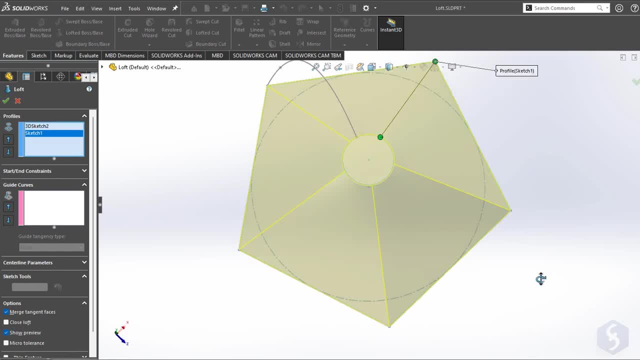 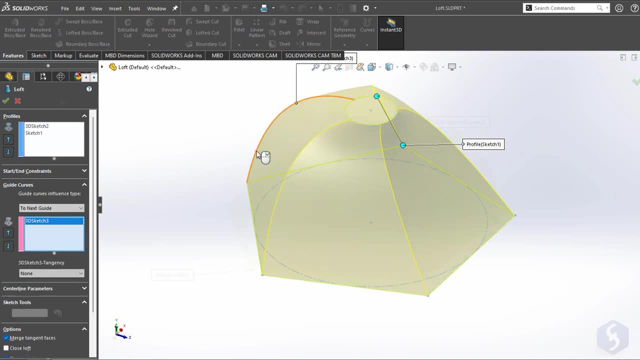 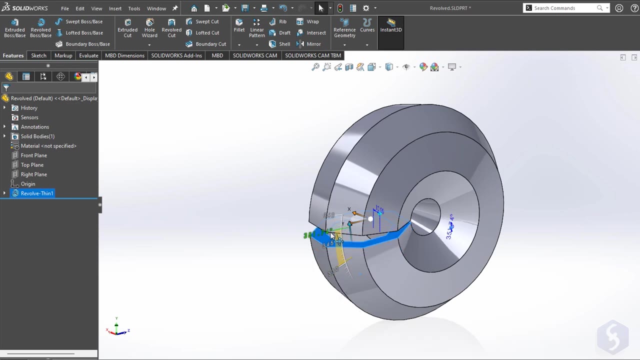 Applying at each step and connecting these in the correct order. There is also the possibility to specify a guide curve in pink color. To edit these 3D features, you can select any face or contour and use the arrows to adjust the extrusion or move these. 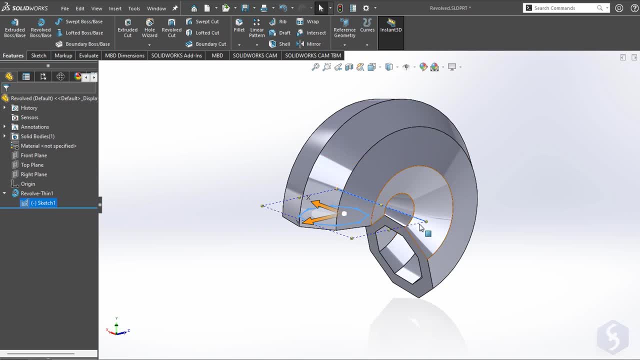 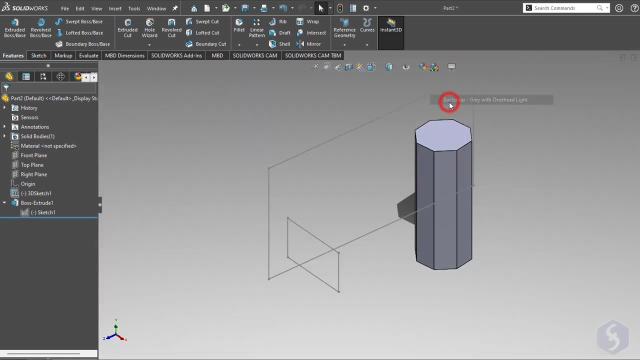 You can also modify the sub-components to reshape the entire object. Solidworks collects several features to render your 3D project. Use Display Style to change the preview mode and apply Scene to set different lights and environment As you finish designing your 3D component. 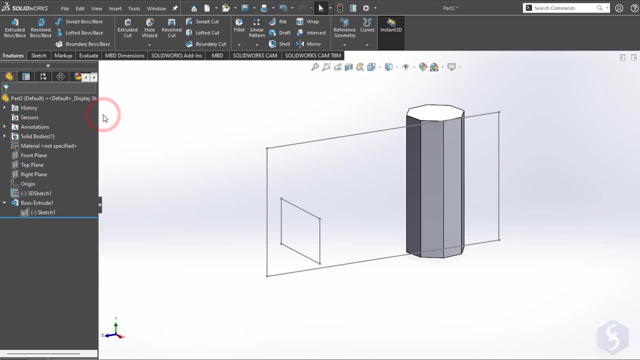 you can save it with File Save As and a sldprt part file. Even if your part project collects multiple sketches and features, Solidworks sees it as a single 3D component. so part of a complete and complex design To join all these 3D components together. 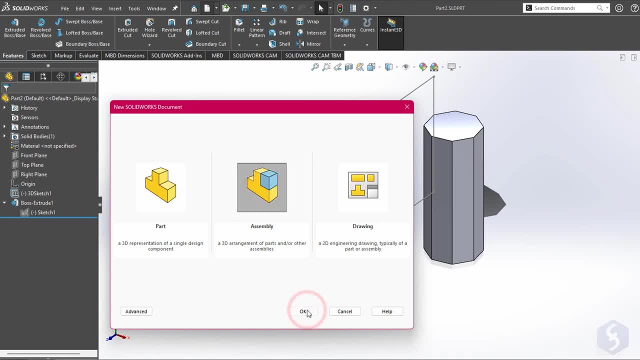 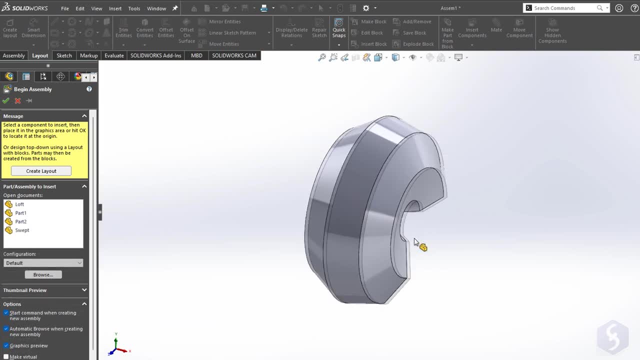 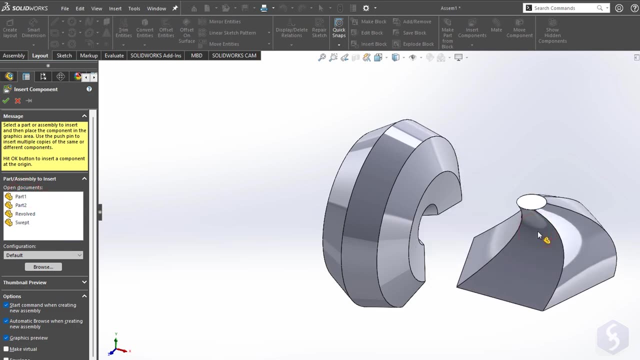 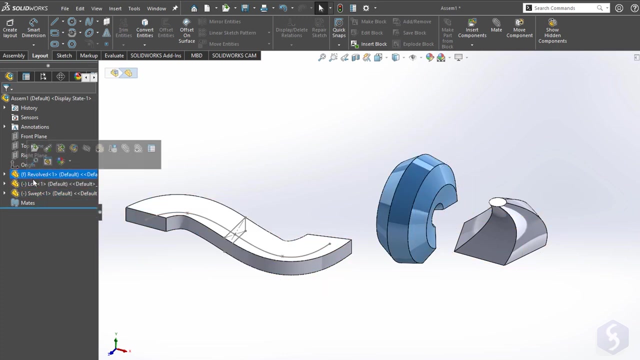 you must open an assembly project by going to New Assembly. At this point import your first component from the left, becoming your main reference. Then import all the others with Layout Insert Component, Except for the reference. you can select any part to move or rotate it. 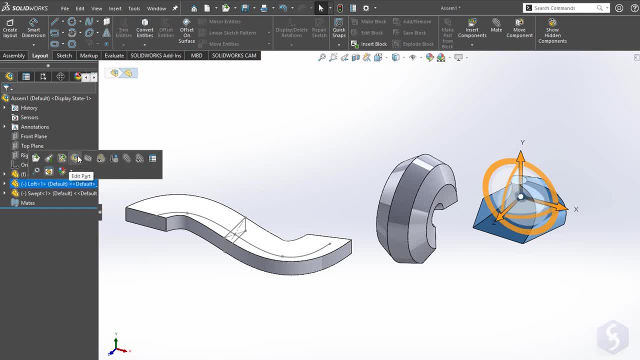 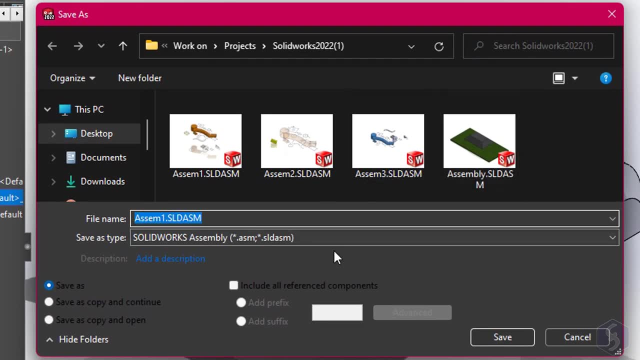 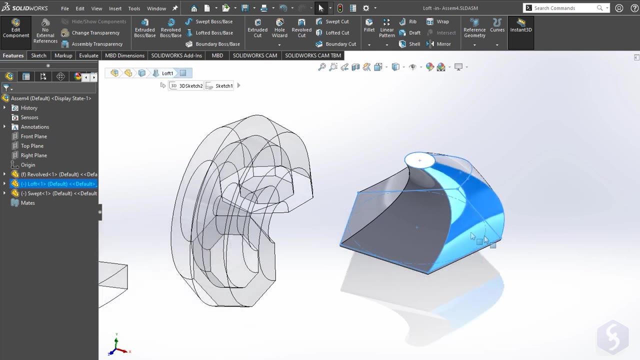 You can also right-click on it and go to Edit Part to modify its features and sketches. The first time you must save your assembly project in a sldasm file. As you finish editing any part, you can return back by right-clicking on the first level. 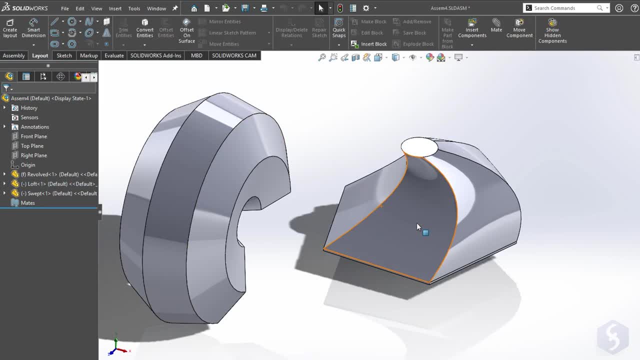 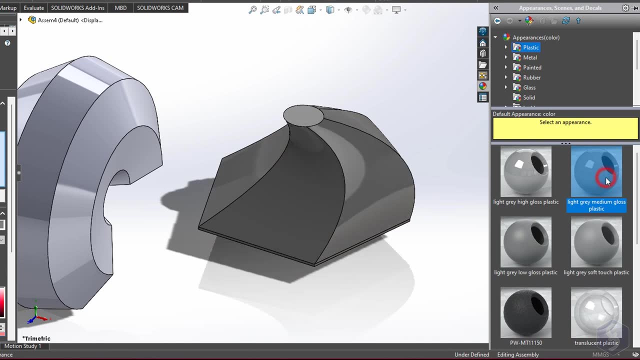 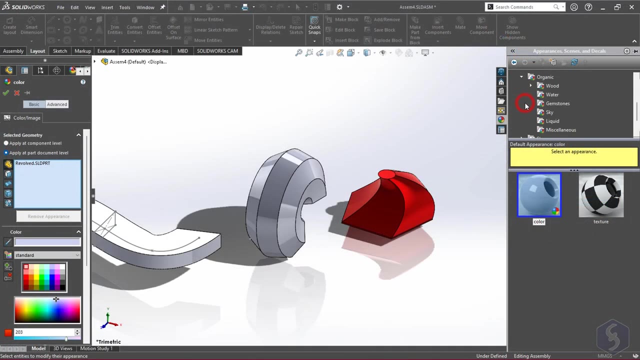 and going to Edit Assembly. Moreover, you can go to Appearances to apply a particular material to the selected part. This affects it entirely and it can't be applied on single sketches or features inside it. This is all. Thank you very much for watching. 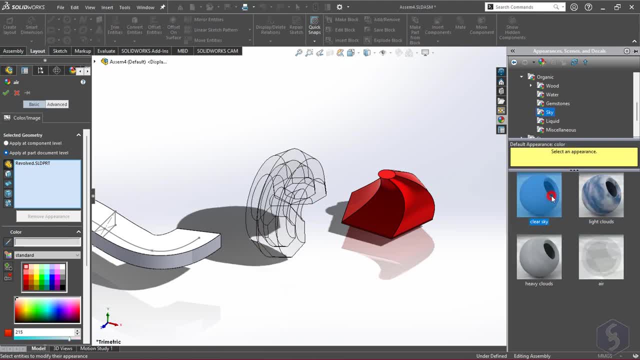 Do not forget to visit our YouTube channel for more amazing and outstanding free tutorials. See you next time.